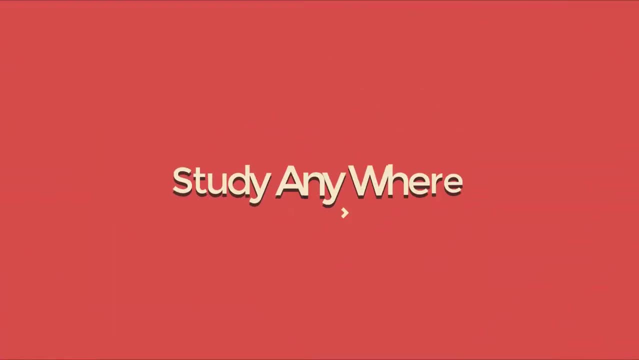 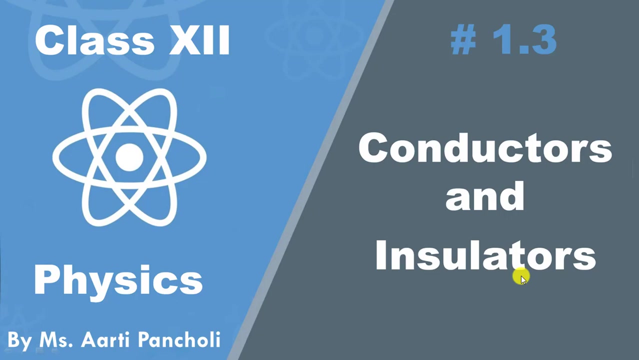 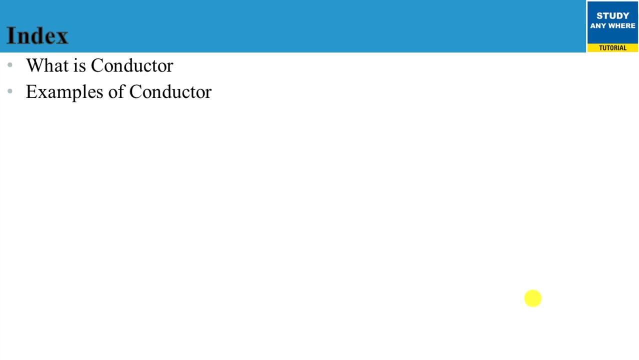 Hello friends, welcome to my physics tutorial channel. In this tutorial, we will learn about conductors and insulators. Today, we will learn the following topics: What is conductor? Examples of conductor. What is insulator? Examples of insulator. Check whether a matter is conductor. 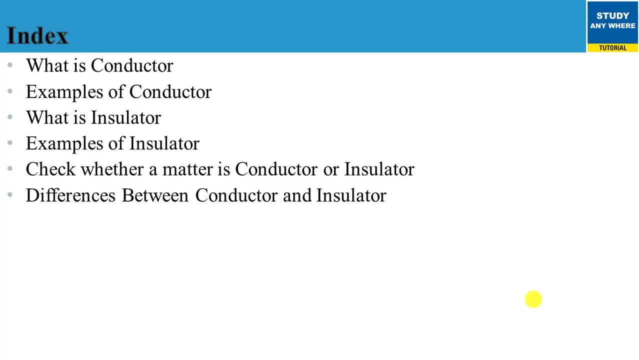 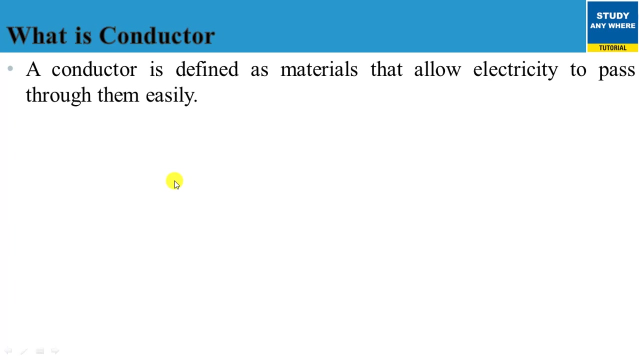 or insulator. Differences between conductor and insulator. What is semiconductors? Examples related with semiconductor. What is superconductor And examples of superconductor? And the last one is exercise: What is conductor? A conductor is defined as materials that allow electricity to 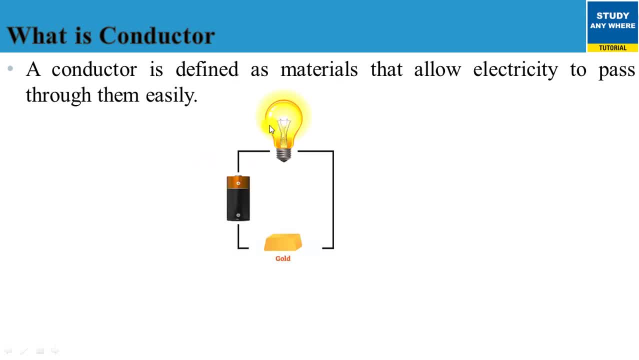 pass through them easily. We have a circuit which is made up with bulb and battery. When we connect them, it allows electricity to pass, because gold is a conductor. The property of conductors that allow to pass electricity is known as conductivity, And the symbol for conductivity is sigma. 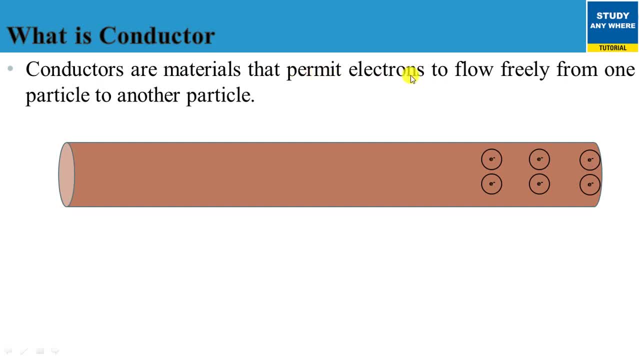 Conductors are materials that permit electrons to flow freely from one particle to another particle. This is a conductor, And electrons are moving from one particle to another particle. The flow of electrons in a conductor is known as the electric current, And the symbol for electric current is capital I When a charge. 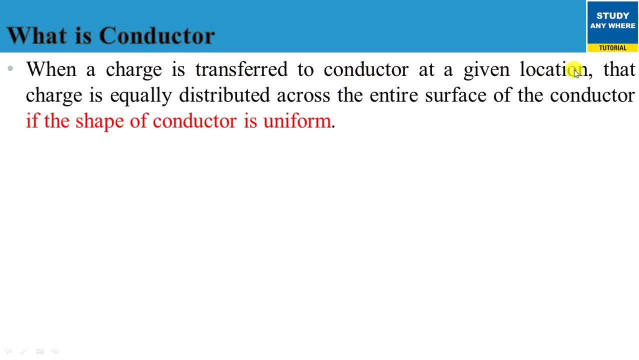 is transferred to a conductor at a given location, that charge is equally distributed across the entire surface of the conductor. But the condition is different When a charge is transferred to a conductor at a given location, that charge is equally distributed across the entire surface of the conductor. 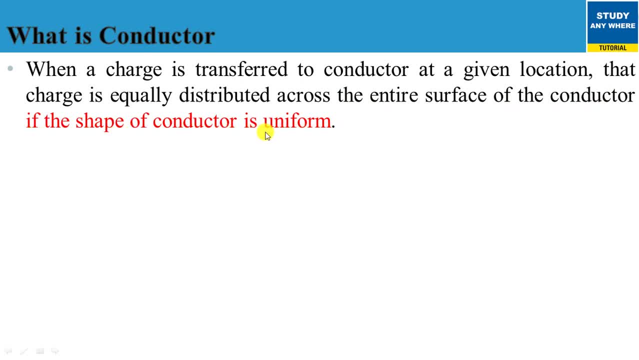 The condition is: if the shape of the conductor is uniform, It is our charge conductor and it is uncharged conductor with regular shape. When charge conductor touch the uncharged conductor, charges will transfer at a particular point. After this, the charge will equally distribute. 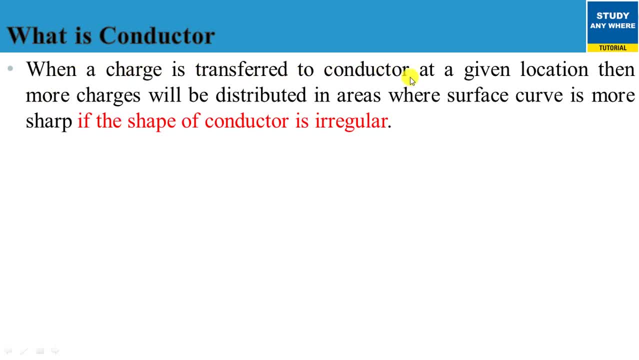 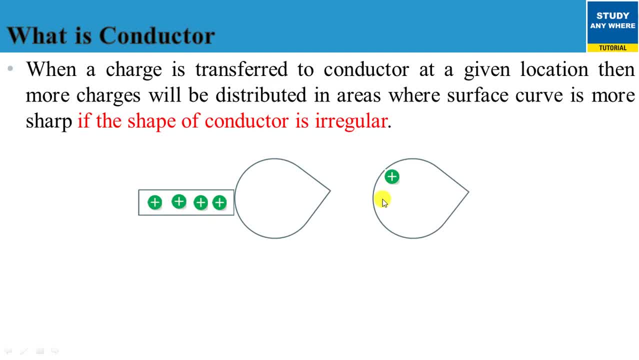 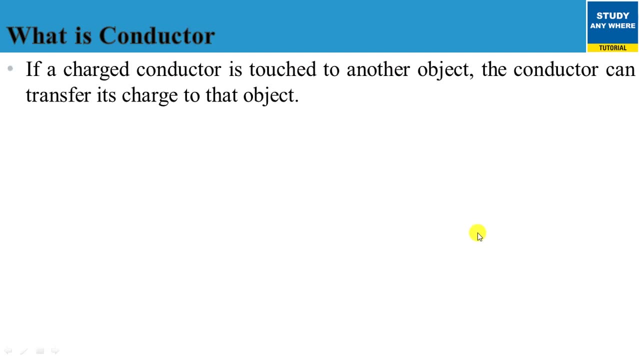 When charge conductor touch the uncharged conductor, charges will transfer at a particular point There wereteam connects. This part has more curve, Therefore more charges will distribute here. If a charge conductor is touched to another object, then the conductor can transfer its. 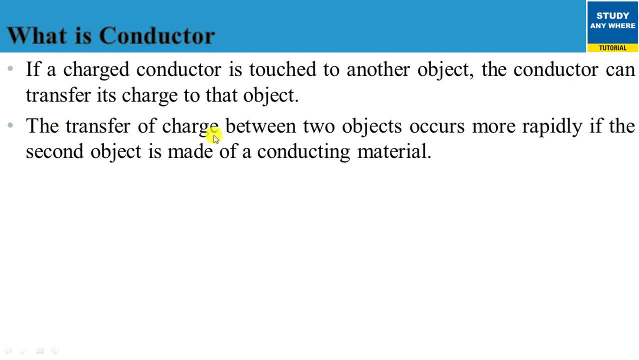 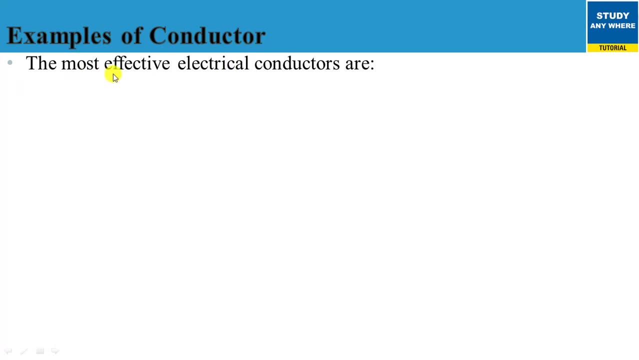 charge to that object. Transfer of charge between two objects occur more rapidly if the second object is made up of a conducting material. Examples of Conductors: The most effective electrical conductors are Silver, Gold, Copper, Aluminium, Steel, Iron, Sea Water, Concrete, Mercury, etc. 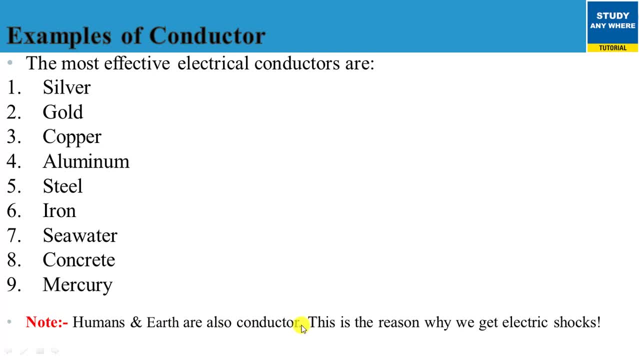 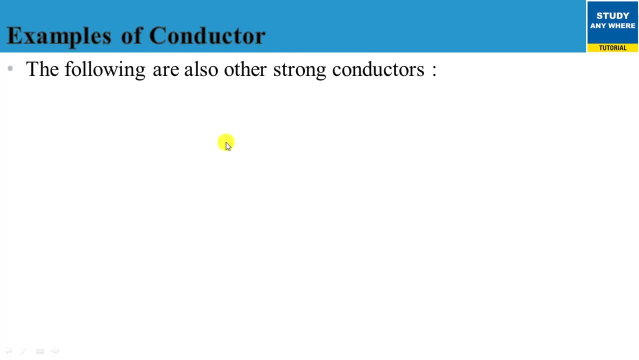 Humans and Earth are also conductors. This is the reason why we get electric shocks. The following are also other strong conductors: Platinum, Brass, Bronze, Graphite, Dirty Water and Lemon Juice. What is Insulin? An insulator is defined as materials that do not allow electricity to pass through it. 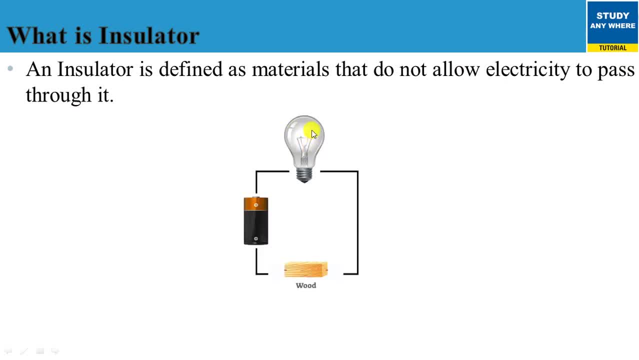 We have a circuit which is made up with bulb and bed. When we connect wood in this circuit, it does not allow the electricity to pass through it, because wood is insulator. The property of insulator that restricts electricity to pass through it is known as resistivity, and the symbol for resistivity is Rho. 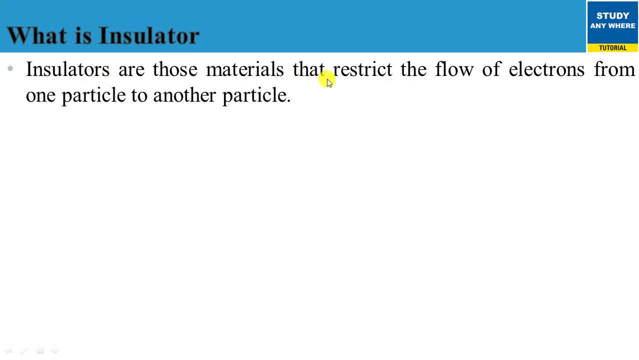 Insulators are those materials that restrict the flow of electrons from one particle to another particle. This is wooden and electrons will not move from one particle to another particle. When a charge is transferred to insulator at a given location, it will not move from. 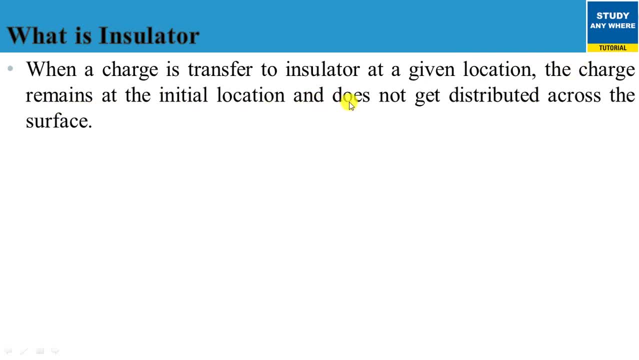 one particle to another particle, The charge remains at the initial location and does not get distribute across the surface. This is our charge conductor and this is an insulating object. When charge conductor will touch to the insulating object, the charge will transfer at a given 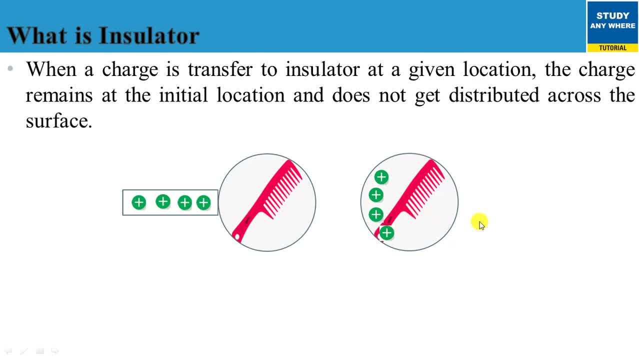 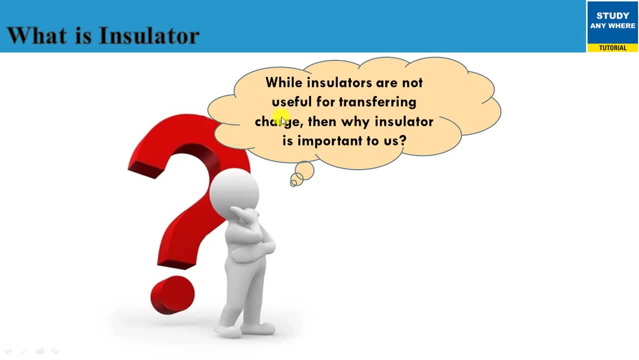 location and will not distribute across the surface, While the charge will not move from one particle to another particle. The charge will not move from one particle to another particle While insulators are not using for transferring charge. then why insulator is important to us? 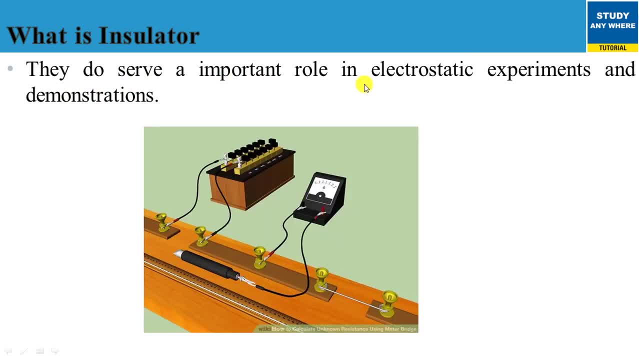 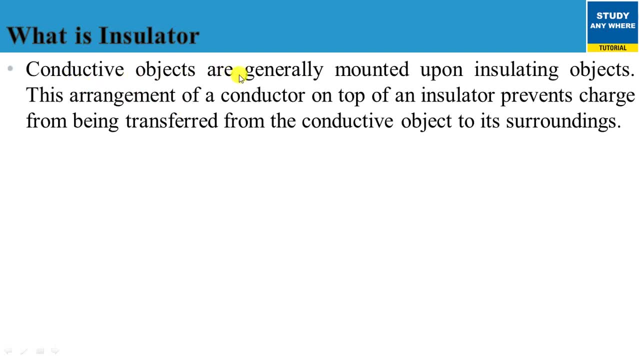 They do serve an important role in electrostatic experiment and demonstration. Conductive objects are generally mounted upon insulating objects. This arrangement of a conductor on top of an insulator prevents charge from being transferred to the insulator. This means charge from being transferred from the conductive object to its surrounding. 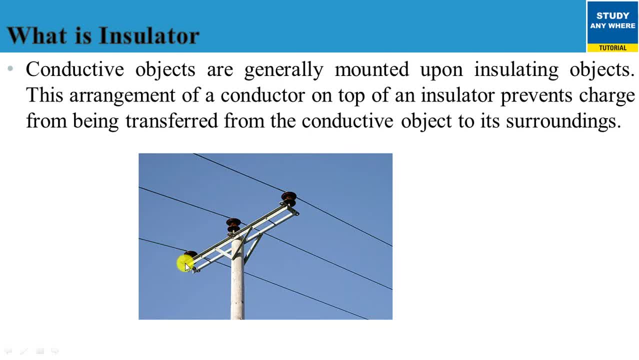 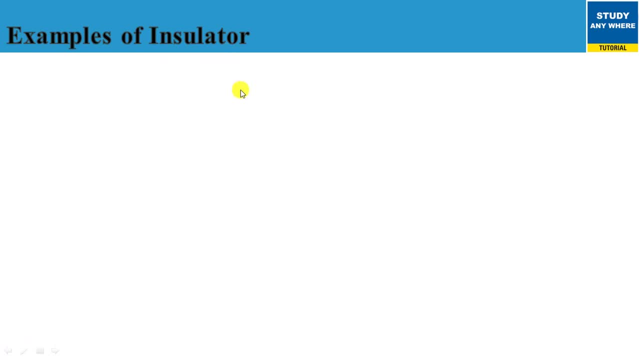 It is an electric pole, It has wire as a conductor and it is mounting point as a insulator. Insulator prevent charge transfer from wire to the electric pole. Examples of insulator: The most effective electrical insulators are Rubber Glass. 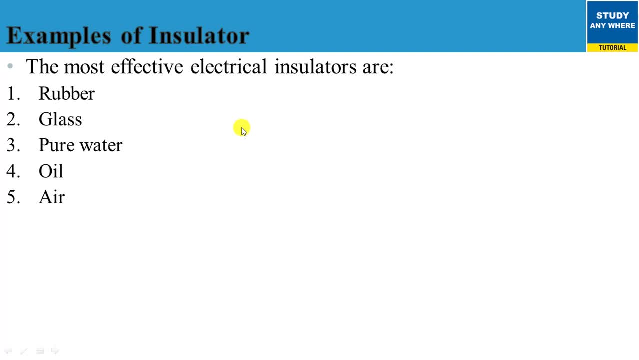 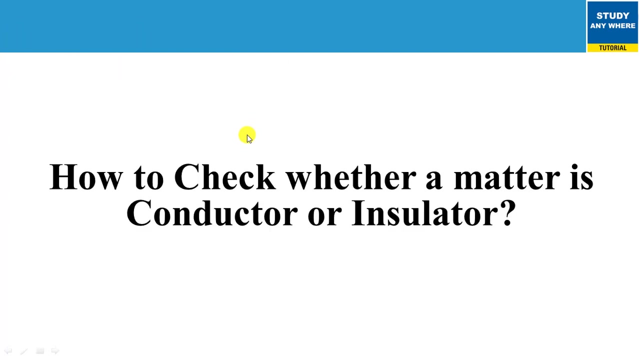 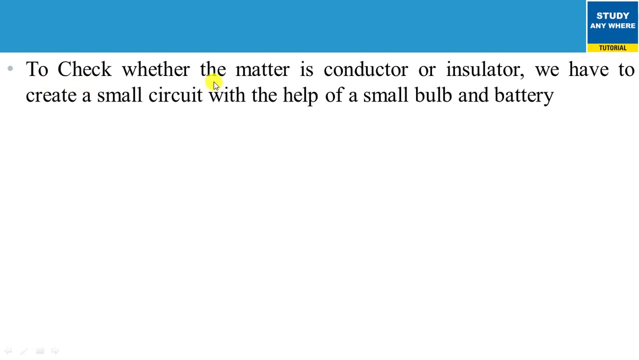 Pure water, Oil, Air, Diamond, Dry wood, Dry cotton, Plastic, Asphalt. The following are also strong insulators like fiberglass, dry paper, porcelain, ceramics, quartz. How to check whether a matter is conductor or insulator. To check whether the matter is conductor or insulator, we have to create a small circuit. 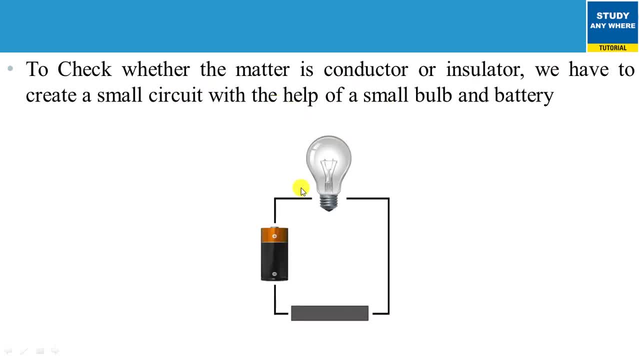 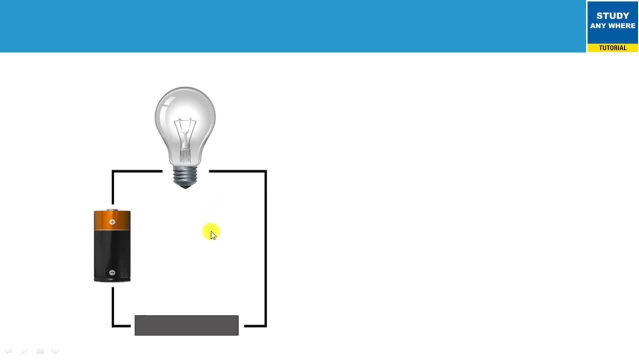 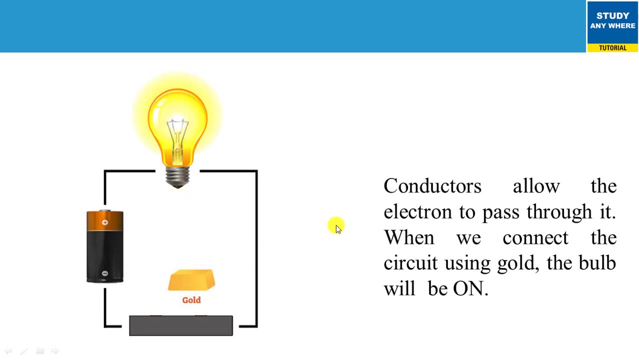 with the help of small bulb and battery. This is circuit which is connected with bulb and battery. When we connect gold in this circuit, the bulb will glow because gold is a conductor. Now, when we connect gold in this circuit, the bulb will glow because gold is a conductor. 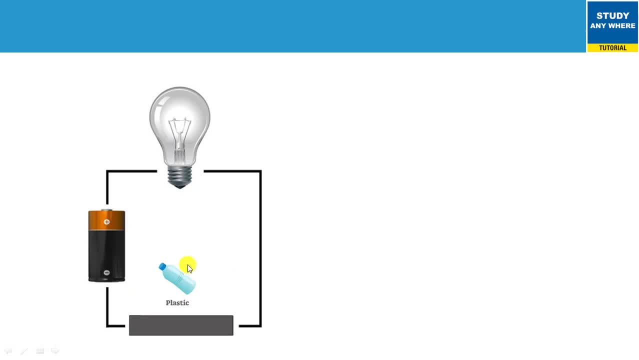 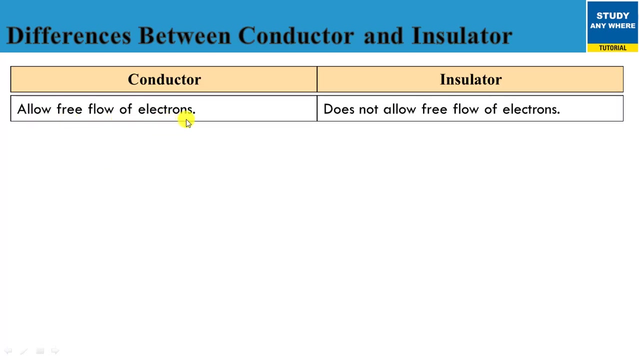 Now, when we connect plastic in that circuit, the bulb will not glow, because plastic is insulator. Differences between conductor and insulator: Conductor allow free flow of electrons, while insulator doesn't allow free flow of electrons. Conductor transfer energy from one form to another form. 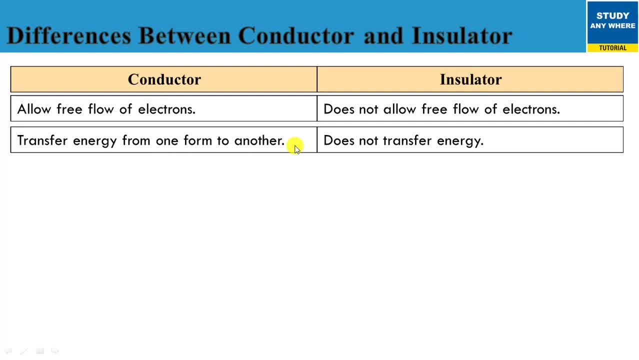 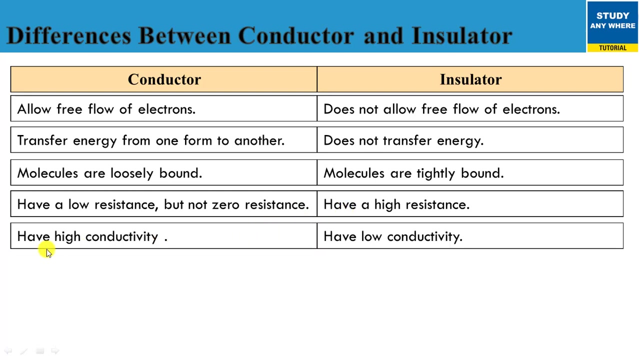 While insulator does not transfer energy. In conductor, molecules are loosely bound, While in insulator, molecules are tightly bound. Conductors have a low resistance, but not zero resistance. In insulator, they have high resistance. Conductor have high conductivity. 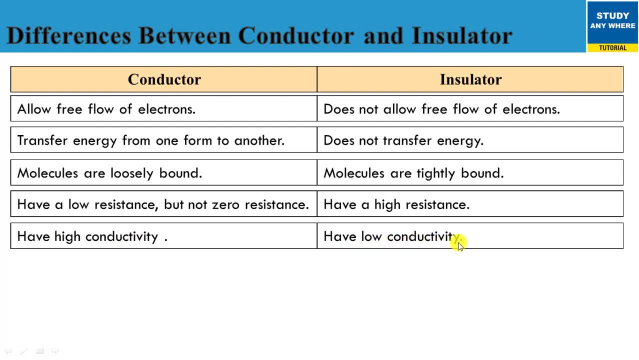 While in insulator they have low conductivity. At room temperature- that is 300 Kelvin, the conductivity of conductor is in the range of 10 to the power 6 to 10 to the power 8.. At room temperature- that is 300 Kelvin, the conductivity of insulator is in the range 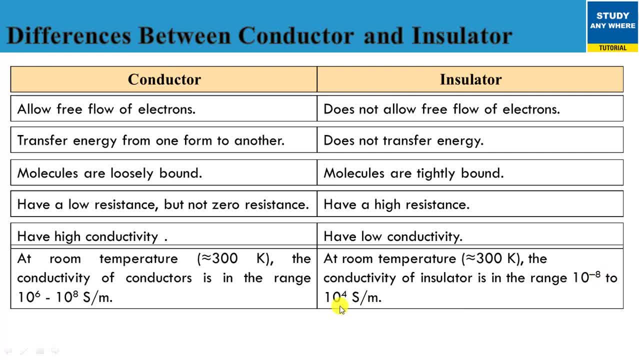 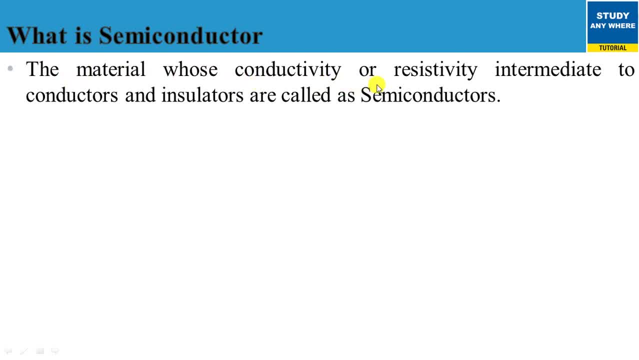 of 10 to the power, minus 8 to 10 to the power 4.. What is semiconductor? The metals whose conductivity or resistance is low, The metals whose conductivity or resistivity intermediate to the conductor and insulators are called semiconductors. 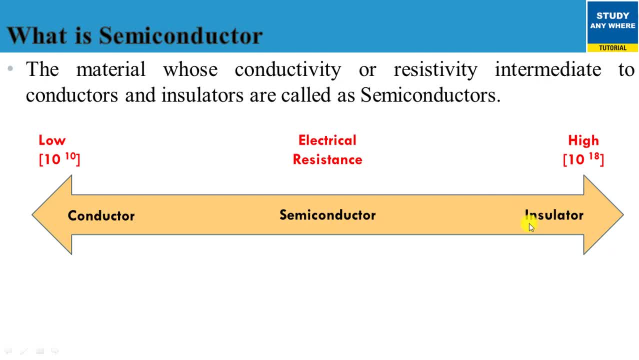 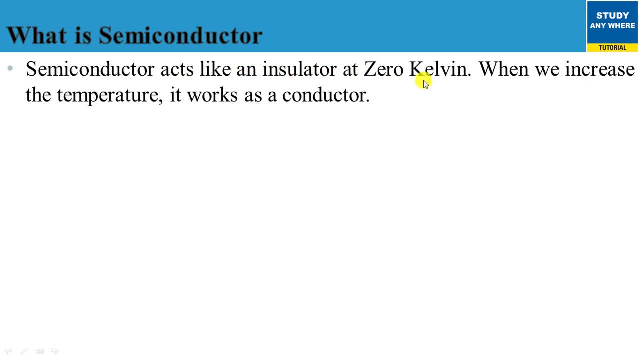 Semiconductor is in between the range of conductor and insulator. Semiconductor act like an insulator at 0 Kelvin. When we increase the temperature, it works as a conductor. Properties of Semiconductor. Semiconductor act like a semiconductor. They have less power loss. 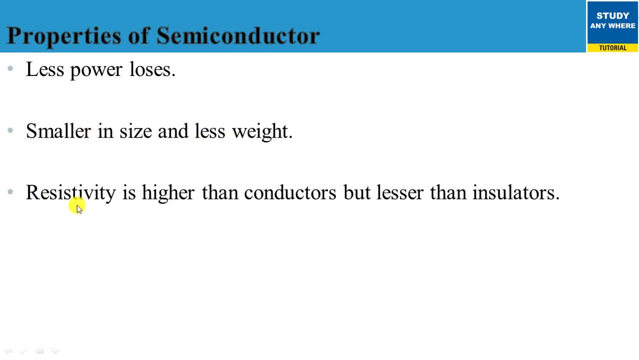 Smaller in size and less weight. Resistivity is higher than conductors, but lesser than insulator. The resistance decreases when we increase the temperature, and vice versa. Type of Semiconductor. There are basically two types of semiconductors. The first one is intrinsic semiconductor. 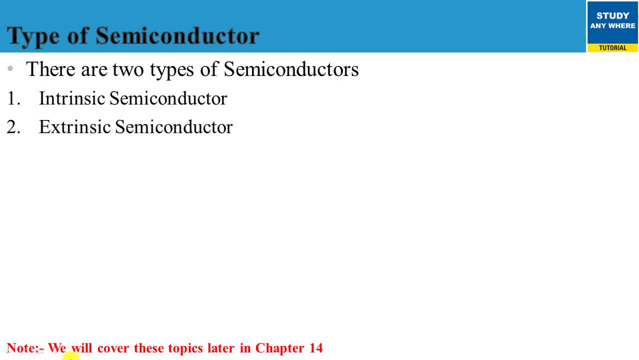 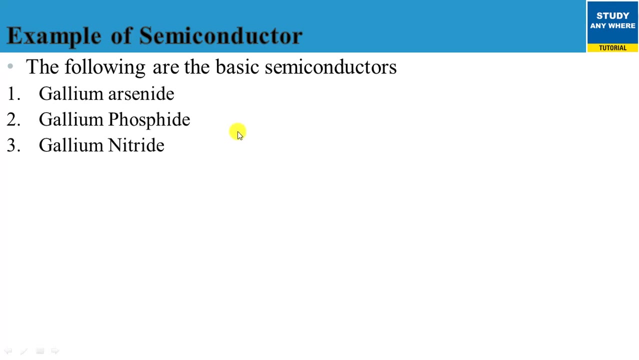 And the second one is Extrinsic Semiconductor. We will cover these above these topics in chapter 14.. Examples of Semiconductor. The following are the basic semiconductors: Gallium Arsenide, Gallium Phosphate, Gallium Nitrate. 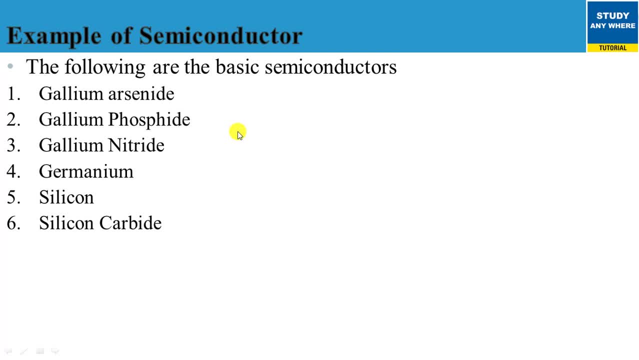 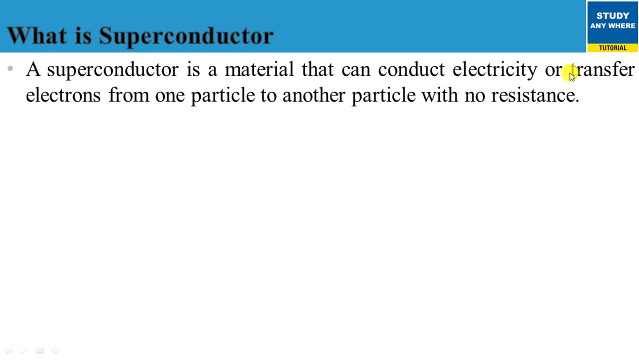 Germanium Silicon, Silicon, Carbide, Lead, Sulphide. Silicon is used in electronic circuit fabrication And Gallium Arsenide is used in solar cell and laser diode, etc. What is Superconductor? A superconductor is a material that can conduct electricity or transfer electrons from one particle to another particle with no resistance. 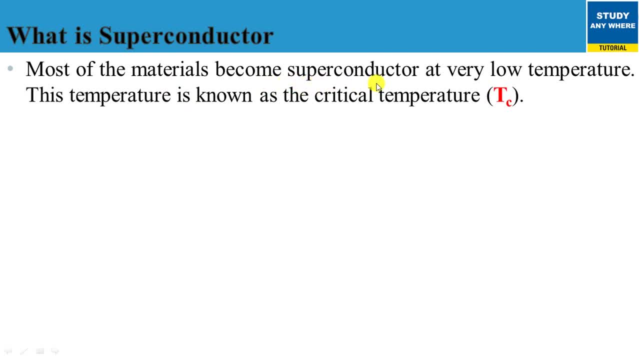 Most of the materials become superconductor at very low temperature. This temperature is known as critical temperature, And the symbol for critical temperature is Tc. Types of Superconductor. There are two types of superconductors. The first one is type I and type II. 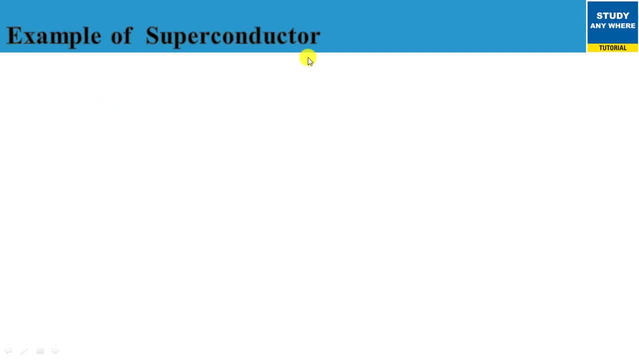 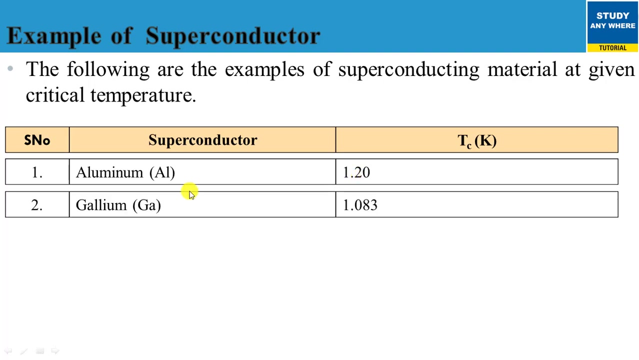 Examples of Superconductor. The following are the examples of superconducting material at given critical temperature. Aluminium: Its critical temperature is 1.20 Kelvin. Gallium: Critical temperature is 1.083 Kelvin. Lithium: 4 x 10 to the power minus 4 Kelvin. 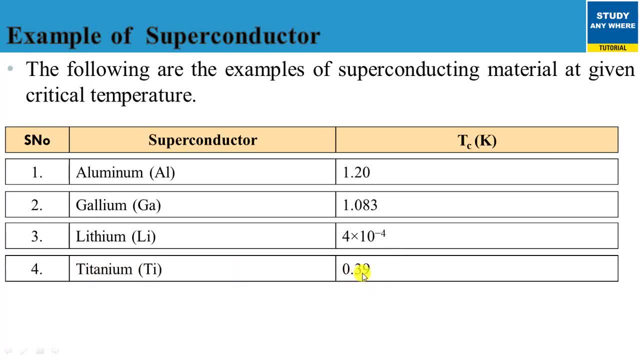 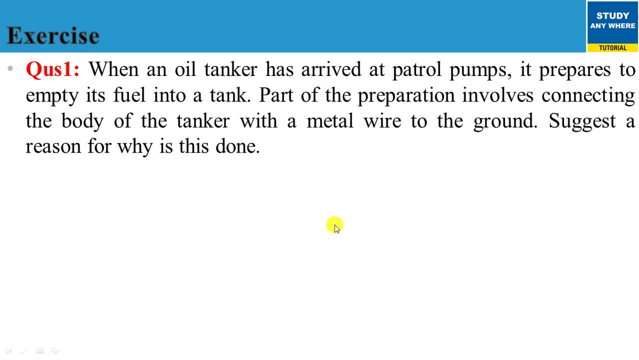 Titanium: 0.39 Kelvin. Zinc Critical temperature is 0.855 Kelvin. Now Exercise Question No.1. When an oil tanker has arrived at petrol pumps, it prepares to empty its fuel into a tank. Part of the preparation involves connecting the body of the tanker with a metal wire to ground.